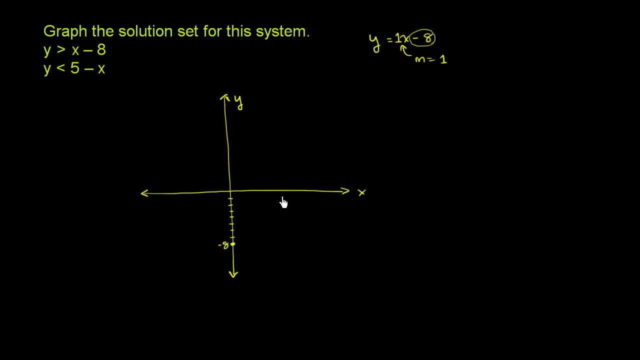 I could just draw a line that goes straight up, or you could even say that it'll intersect if y is equal to 0. If y were equal to 0, x would be equal to 8.. So 1,, 2,, 3,, 4,, 5,, 6,, 7,, 8.. 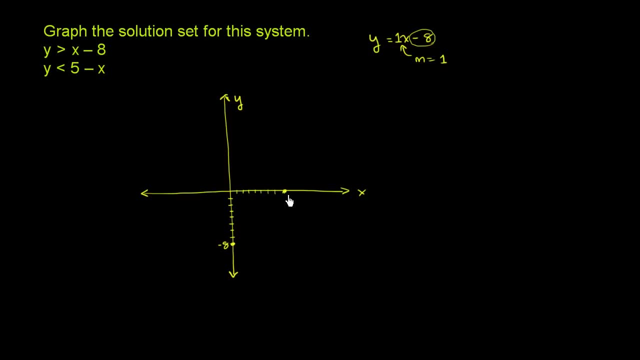 And so this is: x is equal to 8,, but it has a slope of 1.. For every time you move to the right one, you're going to move up 1.. So the line is going to look something like this, And actually let me not draw it as a solid line. 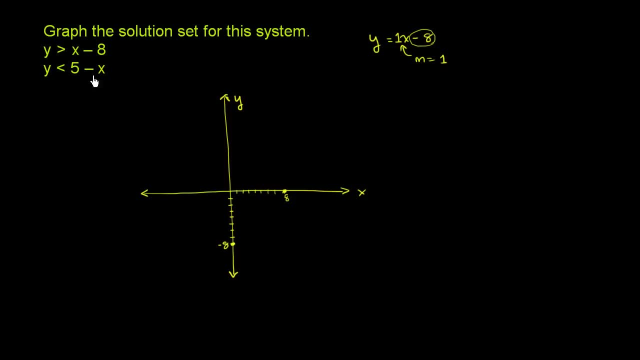 If I did it as a solid line, that would actually be this equation right here. But we're not going to include that line. We care about the y values that are greater than that line. So what we want to do is do a dotted line to show that. 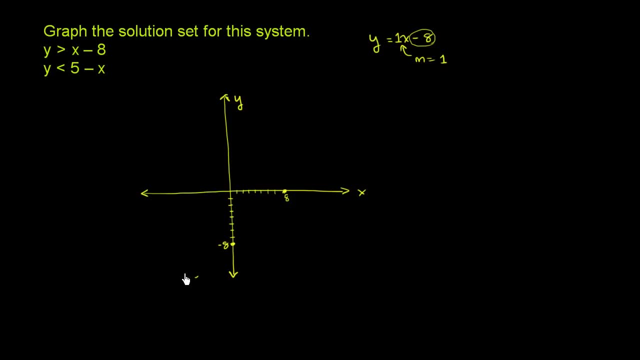 that's just the boundary, that we're not including that in our solution set. Let me do this in a new color. So this will be the color for that line, or for that inequality, I should say. So that is the boundary line. 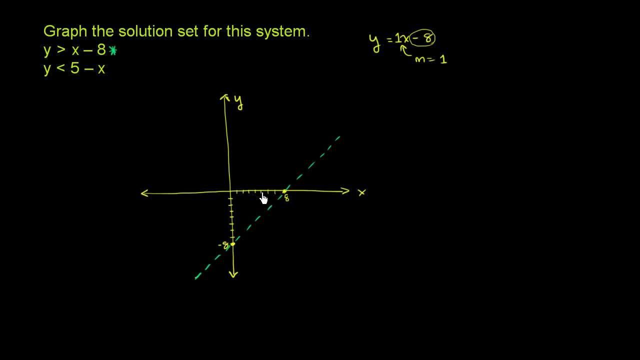 And this says y is greater than x minus 8.. So you pick an x and then x minus 8 would get us on the boundary line, and then y is greater than that. So it's all the y values above the line for any given x. 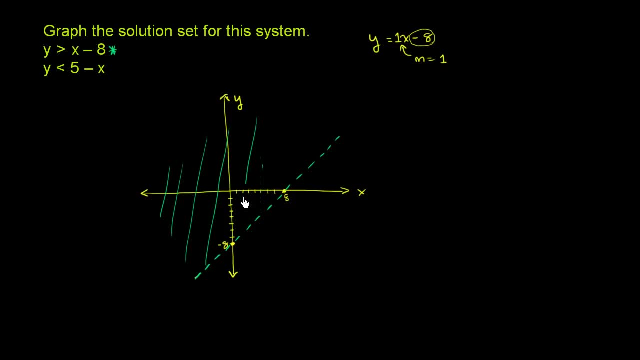 So it'll be this region above the line right over here, And if that confuses you, I mean in general, I like to just think, oh, greater than is going to be above the line If it's less than it's going to be below a line. 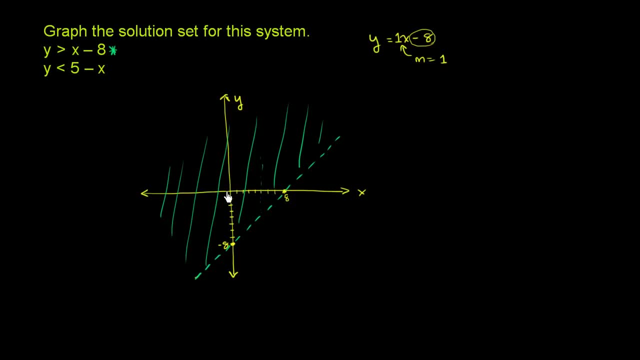 But if you want to make sure, you can just test on either side of this line So you could try the point 0, 0, which should be in our solution set, And if you say 0 is greater than 0 minus 8, or 0 is, 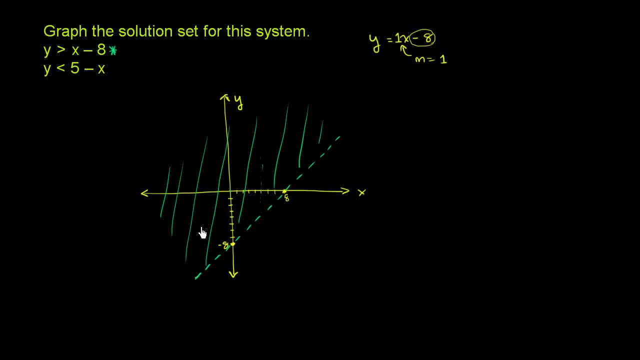 greater than negative 8, that works. So this definitely should be part of the solution set, And then you could try something out here like 10, 0 and see that it doesn't work, Because you would have 10 minus 8,, which would be 2.. 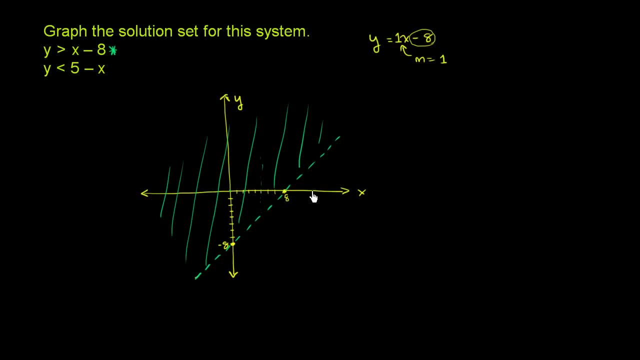 And then you'd have 0, and 0 is not greater than 2.. So when you test something out here, you also see that it won't work. But in general, I like to just say: hey look, This is the boundary line and we're greater than the. 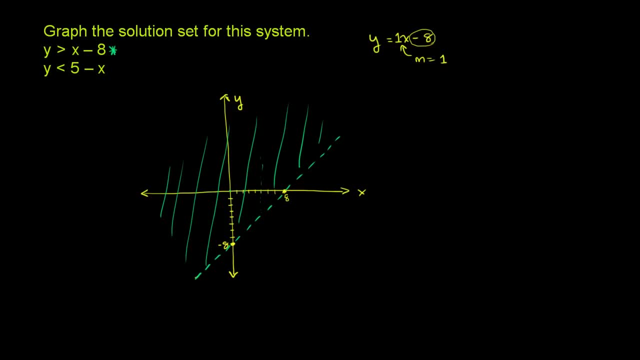 boundary line for any given x. Now, let's do this one over here. Let's do this one. The boundary line for it is going to be: y is equal to 5 minus x. So the boundary line is: y is equal to 5 minus x. 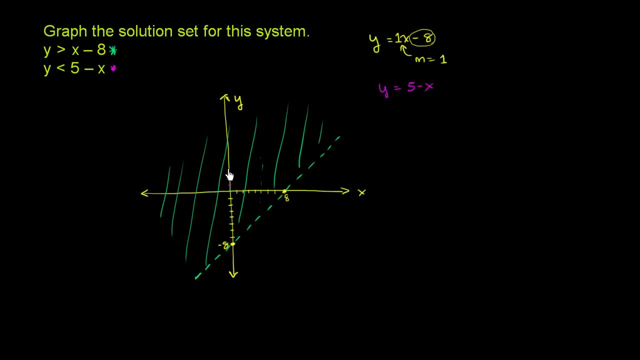 So, once again, if x is equal to 0,, y is 5.. So 1,, 2,, 3,, 4,, 5.. And then it has a slope of negative 1.. We could write this as y is equal to negative 1x plus 5.. 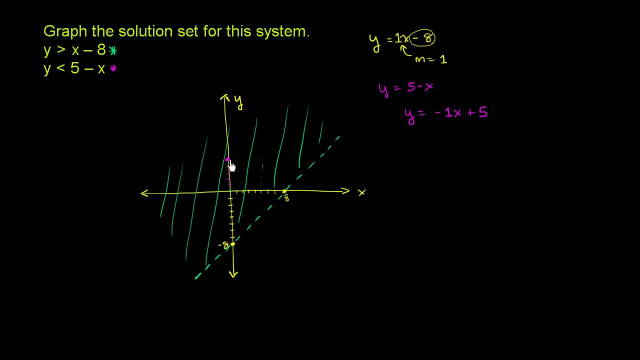 That's a little bit more traditional. So, once again, y intercepted 5.. It has a slope of negative 1.. Or another way to think about it: when y is 0,, x will be equal to 5.. So 1,, 2,, 3,, 4,, 5.. 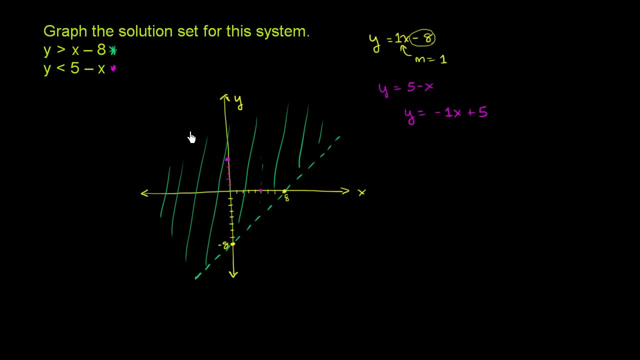 So every time we move to the right one, we go down one Because we have a negative 1 slope. So it will look like this And once again, I want to do a dotted line. I want to do a dotted line because we are: 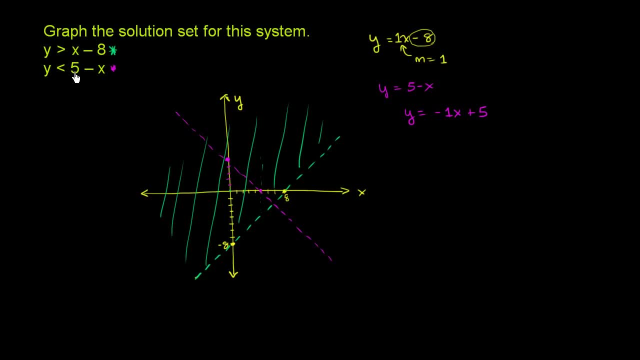 So that is our dotted line, And I'm doing a dotted line because it says y is less than 5 minus x. If it was y is equal to 5 minus x, I would have included the line. If it was y is less than or equal to 5 minus x. 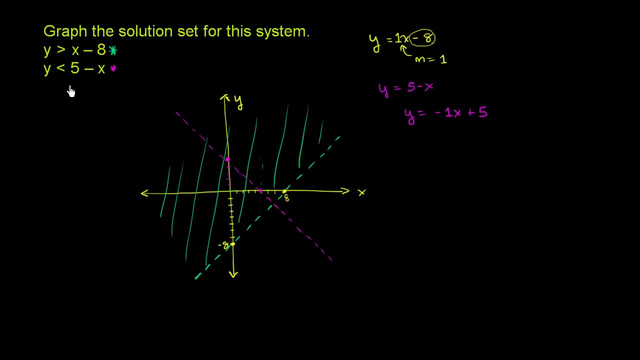 I also would have made this line solid, But it's only less than So for any x value. this is what 5 minus x, 5 minus x will sit on that boundary line, But we care about the y values that are less than that. 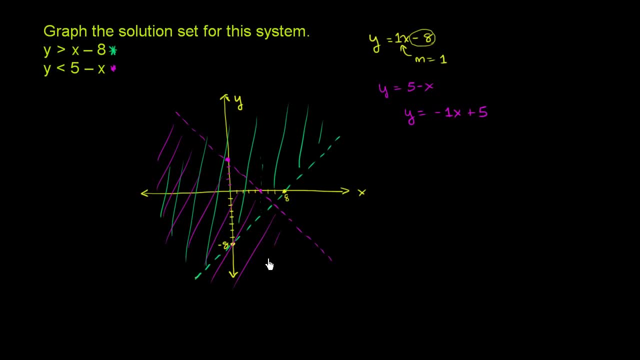 So we want everything that is below the line, And once again, you can test on either side of the line. 0, 0 should work for this second inequality right here: 0 is indeed less than 5 minus 0.. 0 is less than 5.. 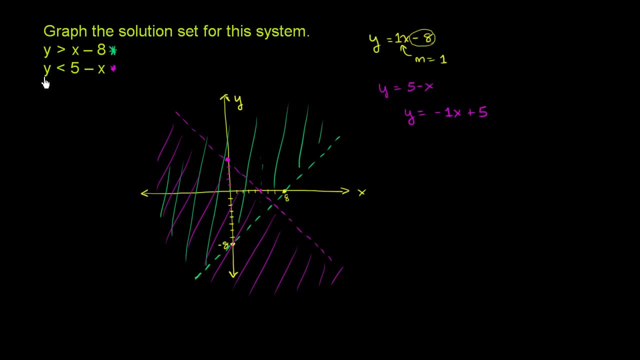 And you could try something like 0, 10 and see that it doesn't work, Because if you had, 10 is less than 5 minus 0, that doesn't work. So it is everything below the line like that And, like we said, the solution set for this system. 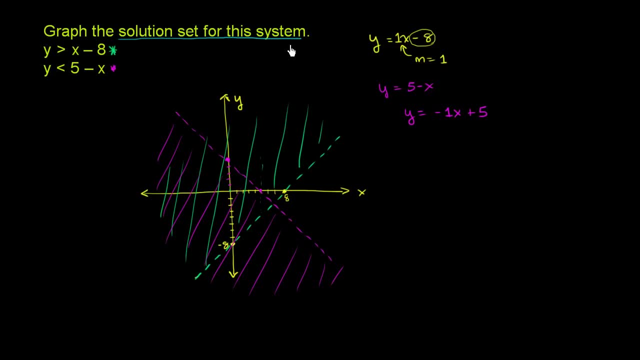 the solution set for the system are all of the x's and y's, all of the coordinates that satisfy both of them. So all the shaded in purple satisfies the second inequality, All the shaded in green satisfies the first inequality. So the stuff that satisfies both of them is their overlap. 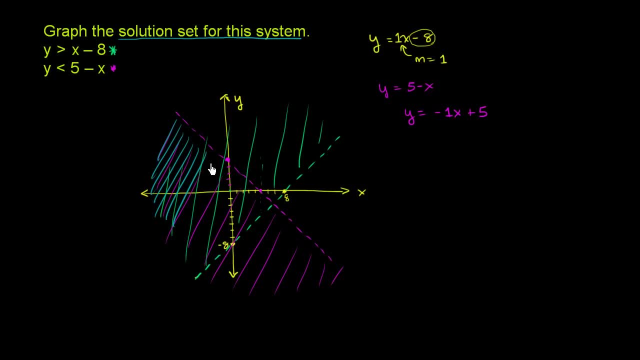 So it's all of this region in blue- Hopefully this isn't making it too messy- All of this region in blue where the two overlap, below the magenta dotted line on the left-hand side and above the green magenta line. That's only where they overlap. 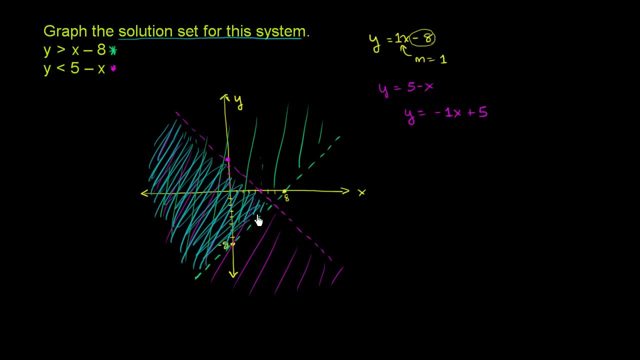 So it's only this region over here And you're not including the boundary lines. 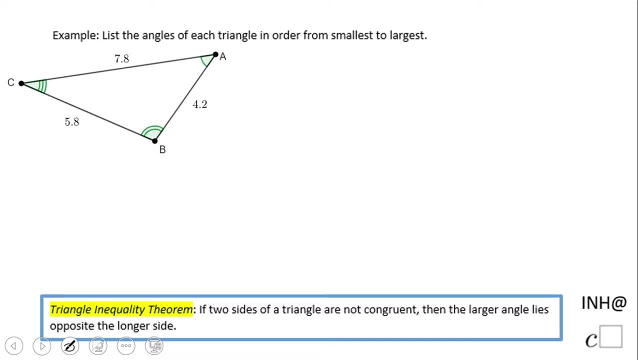 Welcome or welcome back. I need help at C square In this example. here we're going to look to raise the angle of this triangle in order from the smallest to the largest. Okay, and what do we notice here? The sides are gibbered. So for that reason, we're going to use this triangle inequality, TRM, another one which says if two sides of the triangle are not congruent, they are not congruent, then the larger angles lie opposite to the longer side. That's what it says. 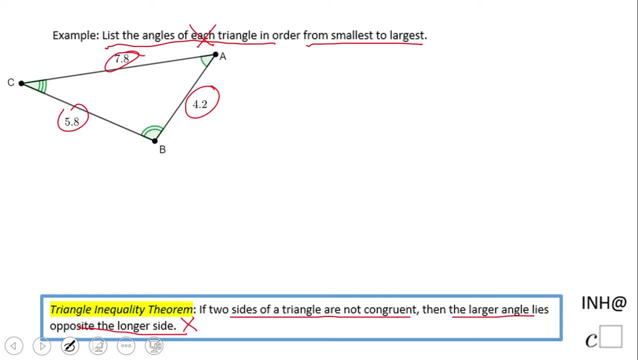 So I'll suggest you to start with the sides, right, If you notice we have here: 4.2 is the smallest one, right, Less than 5.8, and less than 7.8, right, This thing. we can look to the numbers and write it like that: 4.2 is AB, which is less than 5.8, which is BC, which is less than 7.8, which is AC. 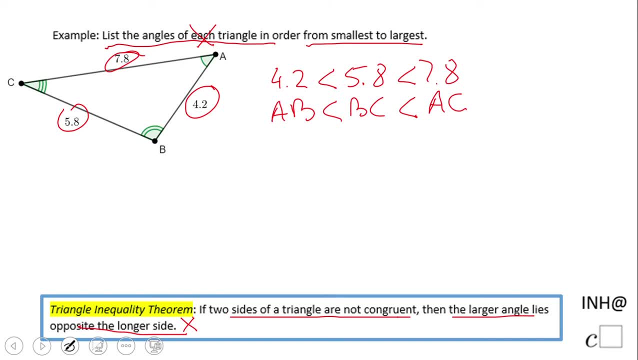 And now we can translate this inequality to the angles using this TRM, as I said, AB. AB is this guy, And the opposite would be angle C, right, So the measure of angle C would be less than what BC is, the opposite of angle A. the measure of angle A. 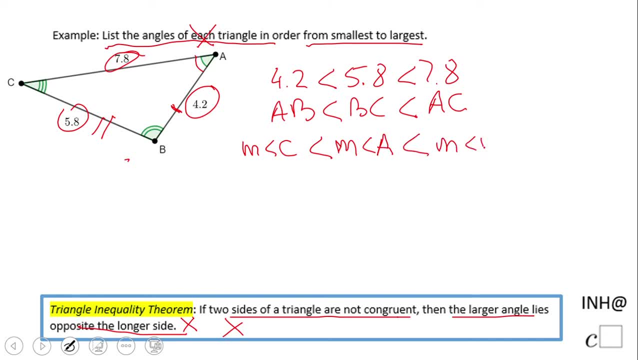 And obviously the last one would be the measure of angle B. This is the way the angles go from smallest to largest, And that's it. If you enjoyed this video clip, don't forget to click the like button And come back on C-squared for more help.